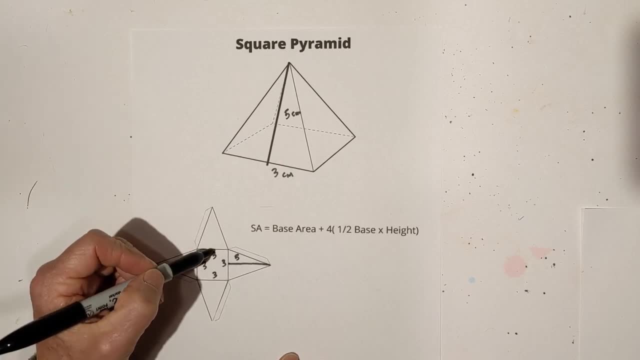 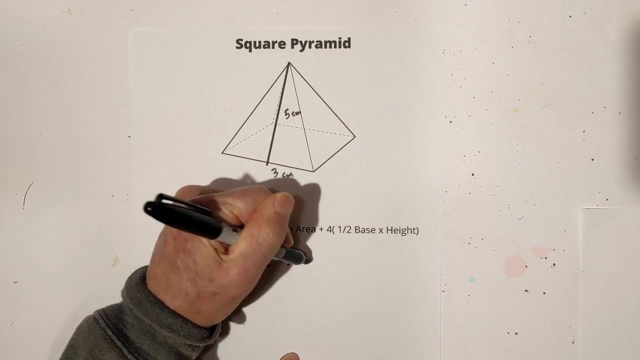 times height is because that's the area of finding of a triangle. Okay, remember, you have height, you have base and then base area is, obviously it is a like a rectangle, and that will be length times width. So let's get started. First, the base area is three times three and that equals nine, and 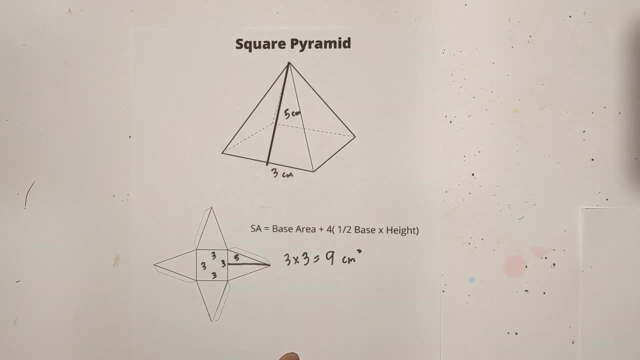 remember it's in centimeters, so that would be centimeters square. Now let's go first. let's go one half base times height. So you have one half times the base and the base is three, and notice that you have four of these. that's why you multiply it by four. So I'm going to go three. 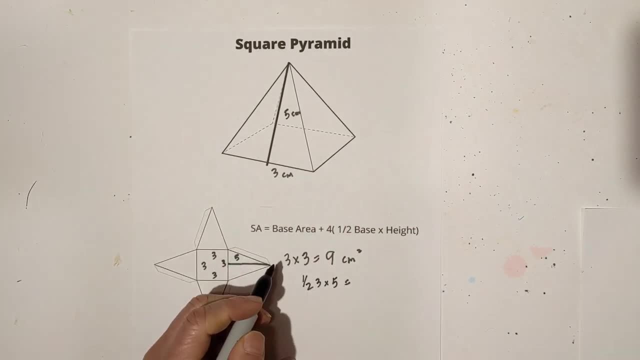 times five and one half times three is 1.5. times five is 7.5 and again that's going to be centimeters square. Now I have to go four times 7.5.. Okay, and the reason again, the reason why we're doing this is that you have four of these, because here's this: 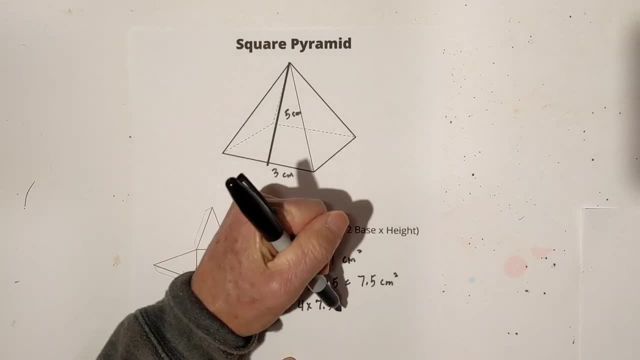 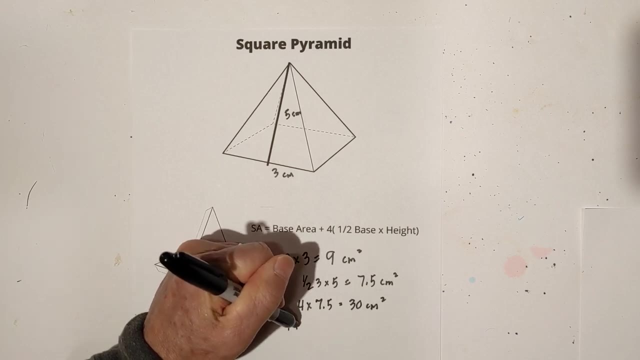 pyramid. if you unfold it So four times 7.5 is 30 centimeters square. So I'm going to add these together: nine plus 30 equals 30 centimeters square, So I'm going to add these together, nine plus 30. 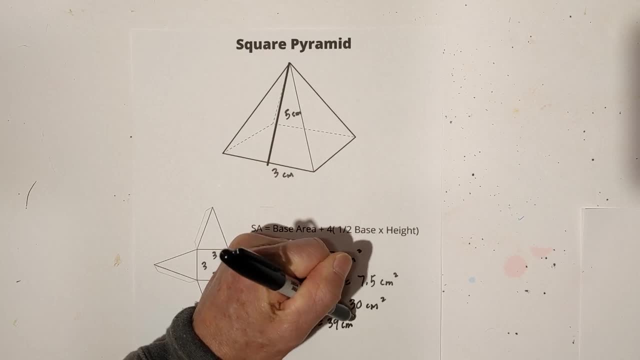 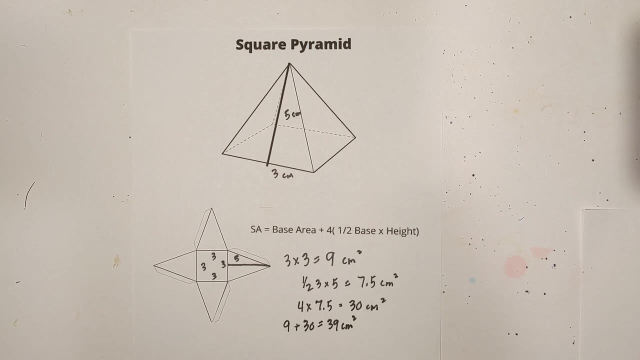 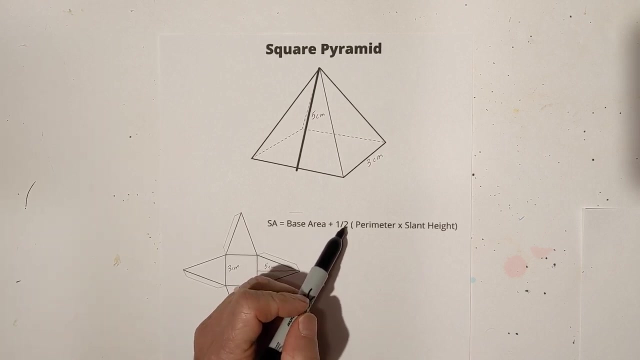 equals 39 centimeters square. Okay, that's technique number one. Let's look at another way to do this. If you would like a different way, you can try this. It's base area equals one half times the perimeter times slant height. So let's work through that, Okay. first we have base area. 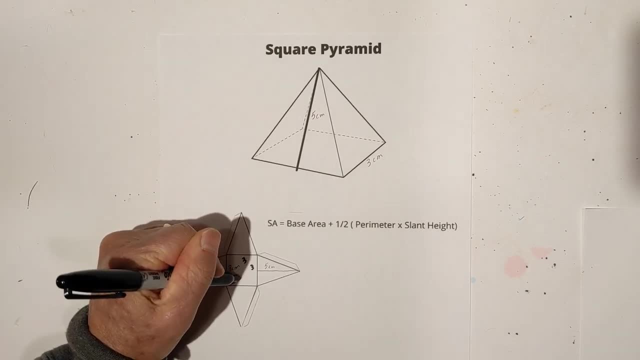 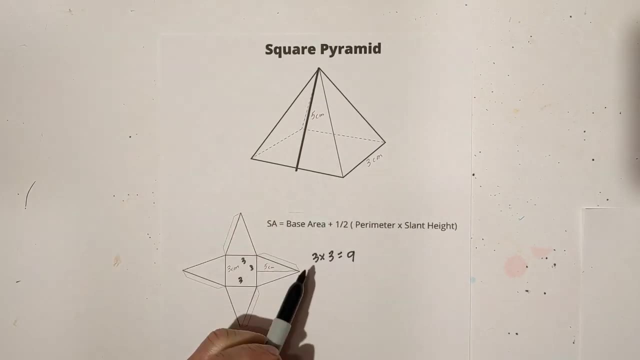 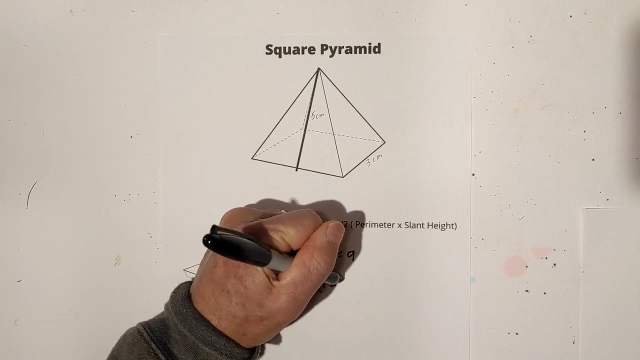 Remember, it's a rectangle. Each of these are three, So you have three times three, which equals nine. Now we're going to add this to one half times the perimeter times slant height. Well, the perimeter is 12.. 3, 6, 9, 12.. Okay, so let's go 12.. So it's going to be one half times twelve plus, and you know the slant height is five. 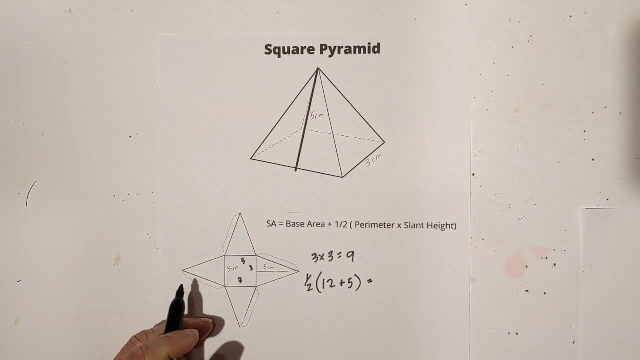 When you multiply this together, it is twelve, not plus 12.. excuse me, it is 12, not plus 12 plus, and you know the slant height is five. When you multiply this together, Excuse me, it is 12, not plus 12..